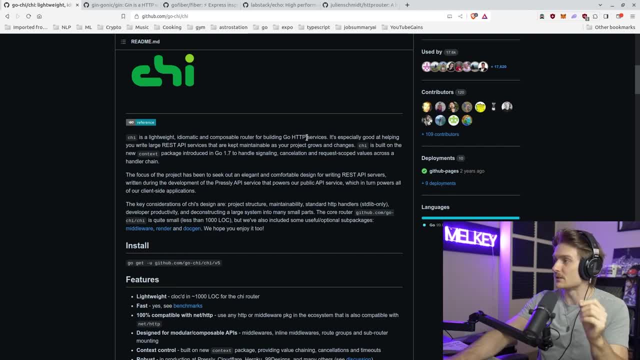 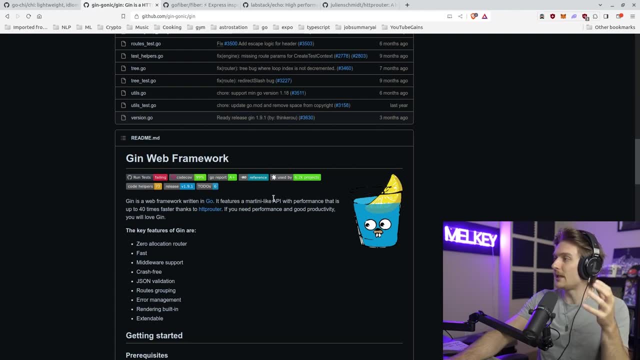 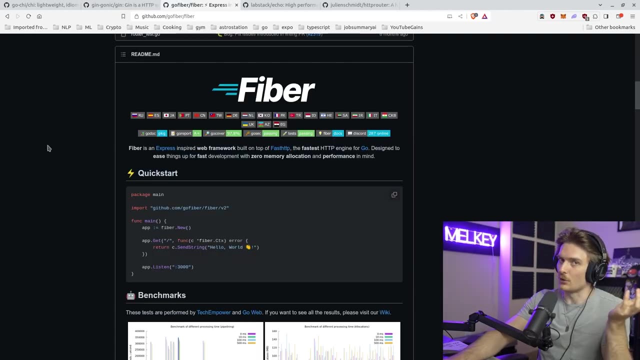 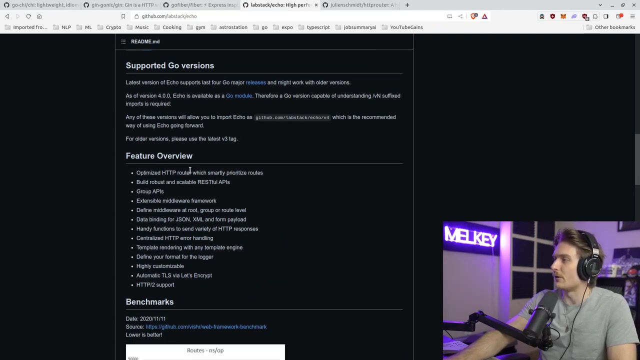 idiomatic and composable wrapper. And if I just read the first bit of the readme, Chi isn't, And I've actually previouslyικniiv eências forcke feature overviews. optimize hp router with smartly prioritized routes. build robust and scalable. restful apis. have you noticed a pattern? you see a lot of these libraries in go. these frameworks are essentially doing the same thing. they are just wrappers on top of the standard library that go offers, and this isn't necessarily a bad thing. and i'm not saying all of these are the exact same. 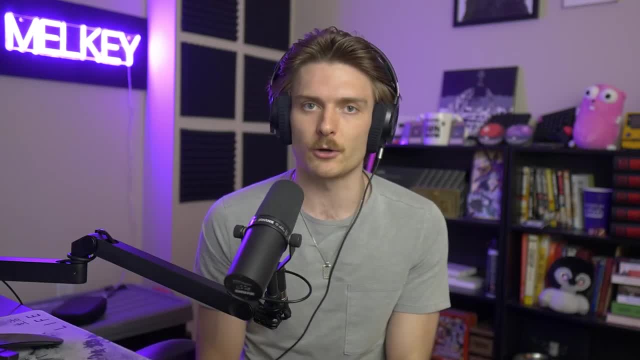 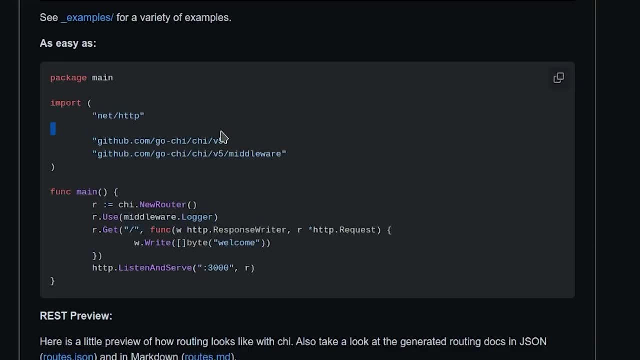 but when you are focusing on just creating routes or middleware or anything like that, you can pick any of them. here we're back on go chi and you can see this example as easy as you have your imports. so there's chi, there's a standard http library and there in your function main, you. 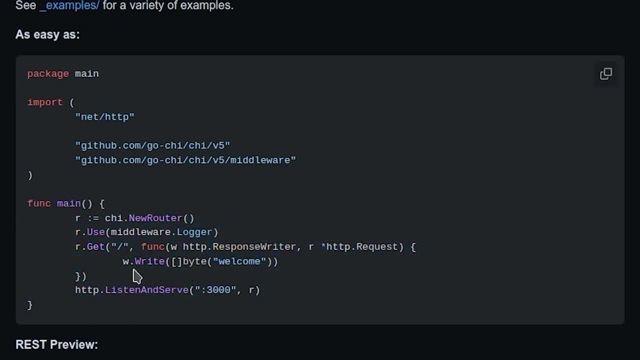 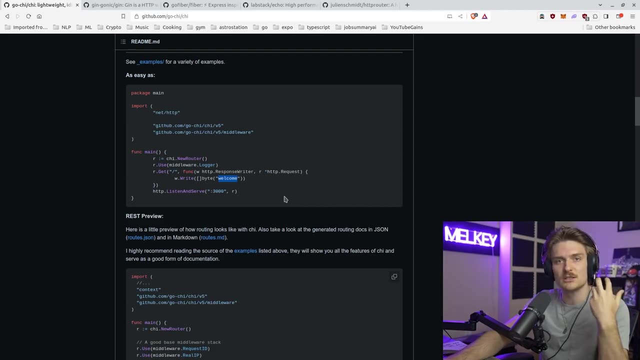 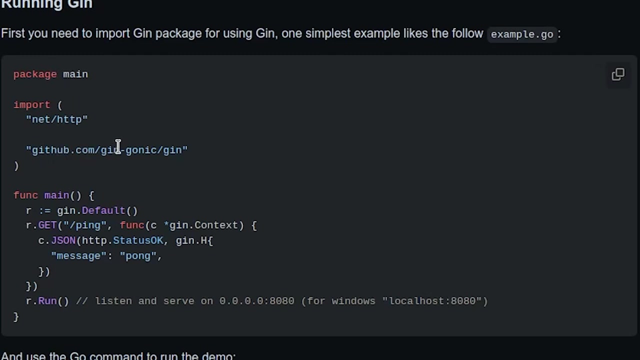 create your new router using chi library. you create some middleware and you're designing a route here. this get route with a response that just says welcome looks super simple. wow, chi is great. all right, let's flip on to gin. for a second gin, you have your imports, net http and gin. okay. 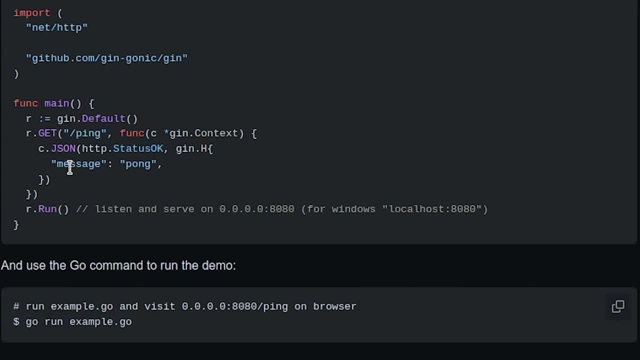 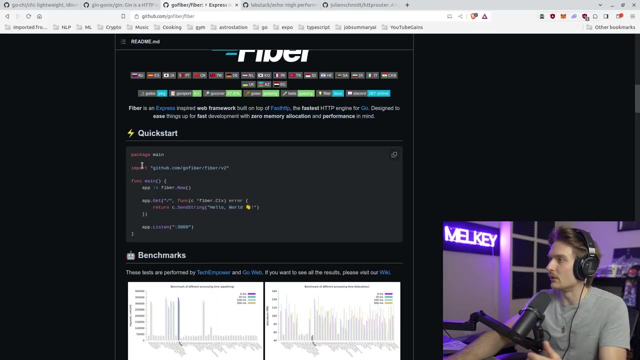 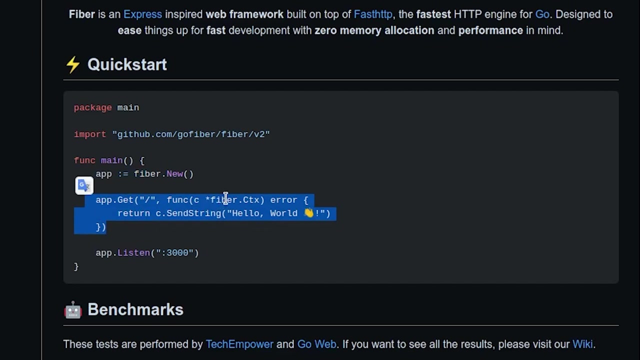 awesome. so you create ginhtml default and, oh, you define your route that has a response: okay, cool, this is great, this is awesome. how about we check out fiber for a second? you have your import fiber and oh oh, app fibernew and you define. this looks almost exactly the same. you have your get route that just says hello world. 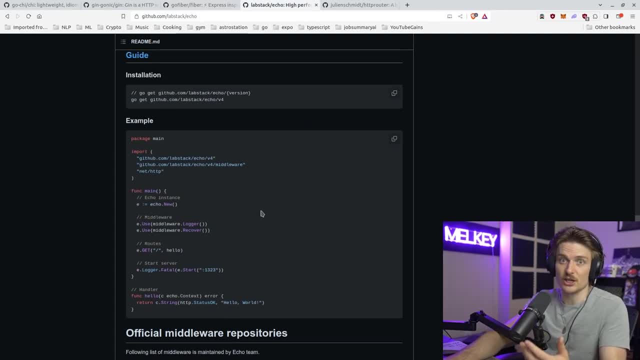 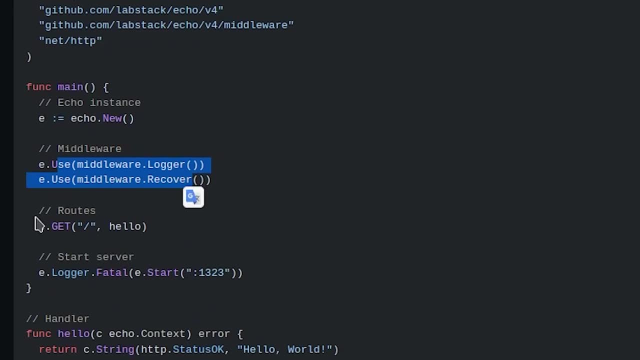 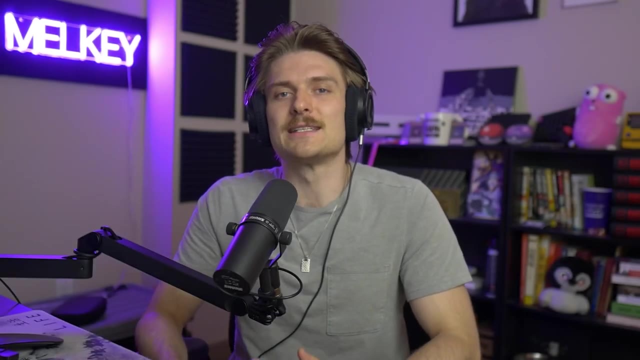 okay. well, how about we check out echo for real, quickly, just you know, just to check it out? how different can it be? and oh, you create your new echo instance- okay, middleware or all right- and you get route with a response that says: hello world. you can see that all of them follow the. 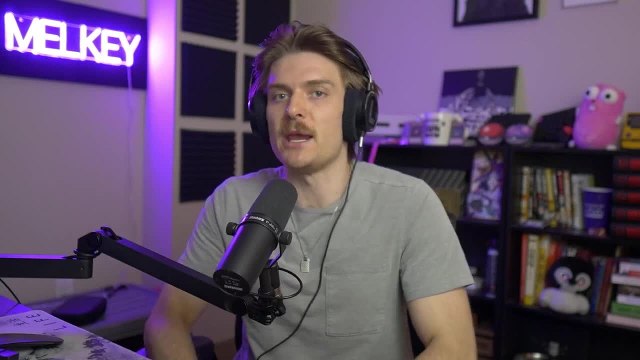 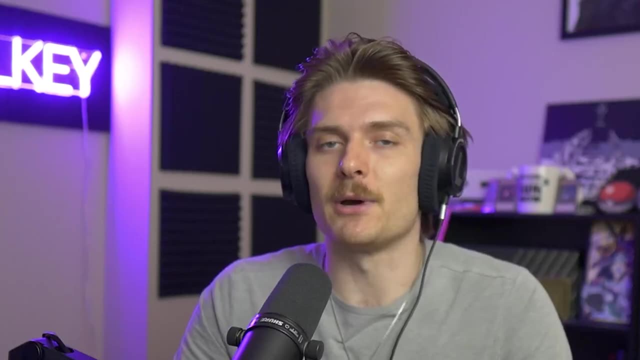 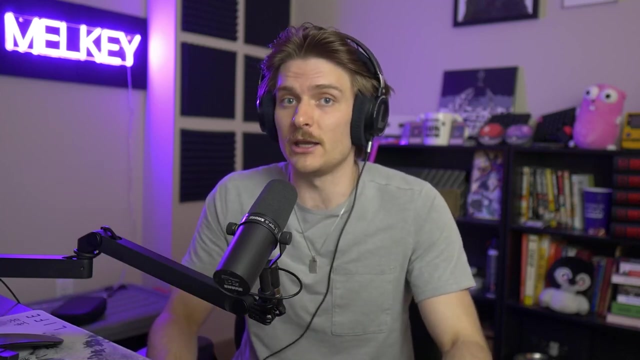 same pattern and, yes, jin and chi may have things that provide more use case in a fully fleshed out library and framework to use, but at the end of the day you create the instance, you define your get or post route and you pass it a function or literally a json payload and it just does what you tell it. 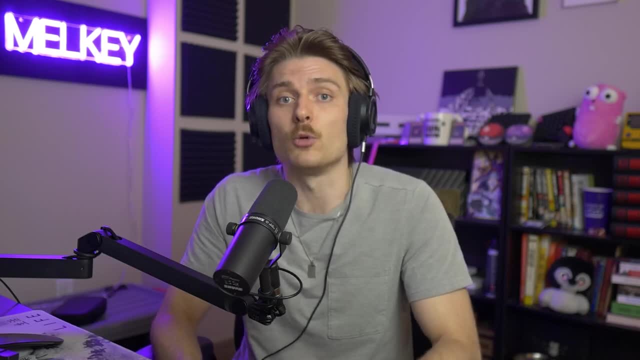 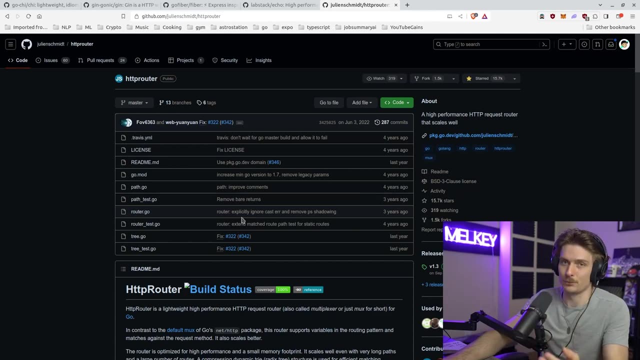 to the handler, respond to the route. how you do it, and that's how you create your get route and you define it, and it looks the exact same way for every single one. and just to showcase another example, one that i personally recommend is http router by julian schmidt, because this is the closest. 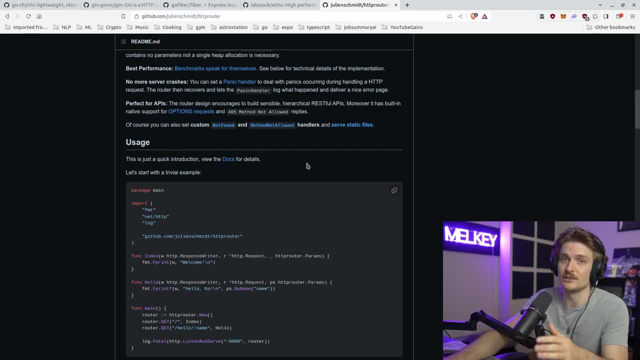 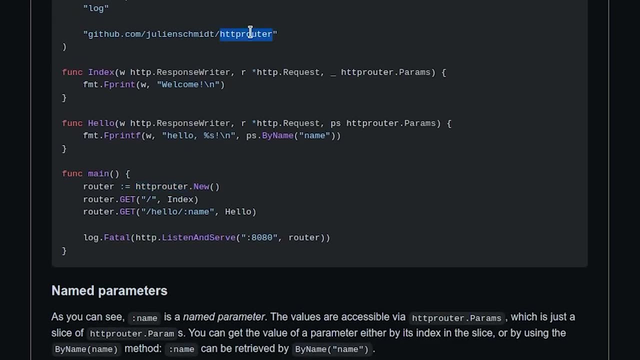 to the standard library that you can get between all the examples i previously showed. you can see here. you define two handlers, index and hello. define your routes by instantiating http router from the library they pull in and then you have a two dot get math methods on these two routes. 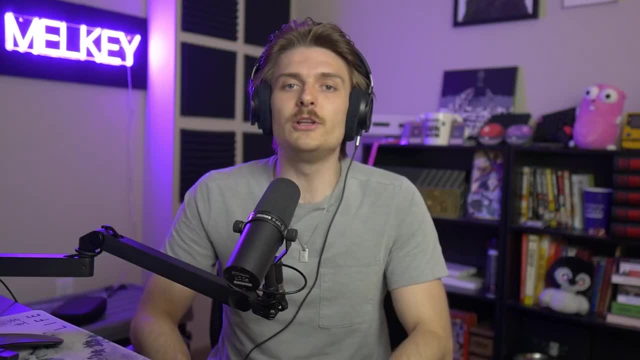 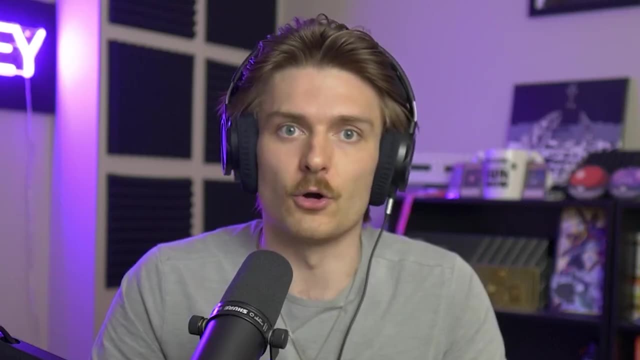 declared and they will pass the function of the handler, and so that's how you define your get route. and so what i really want to kind of convey, and what i always talk about when i explain go to someone, is that you have to separate your thinking of go from javascript. if you're coming from that, 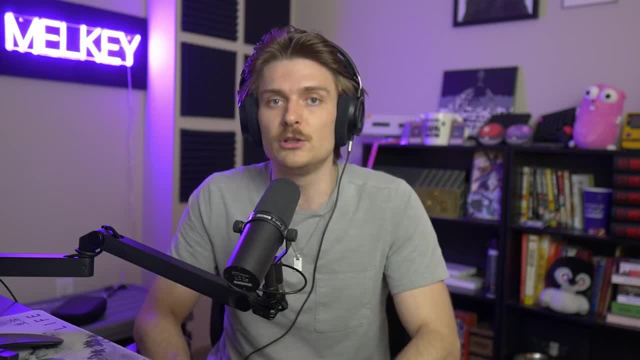 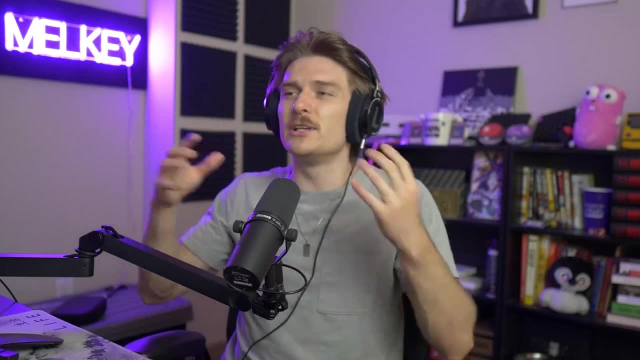 world or any other world, because go you can truly do everything with the standard library. go is in that program language where you should be picky and really pulling resources or deciding which framework is right for you. of course, you can use particular use cases that you can read about and 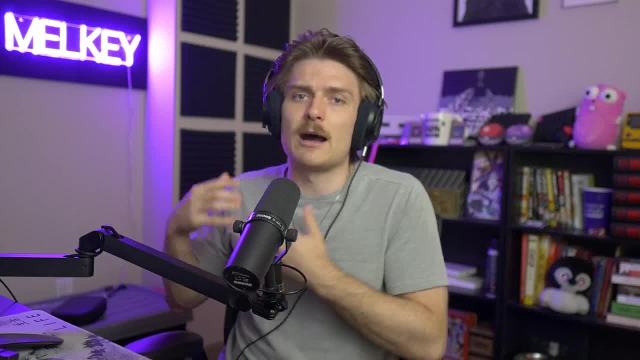 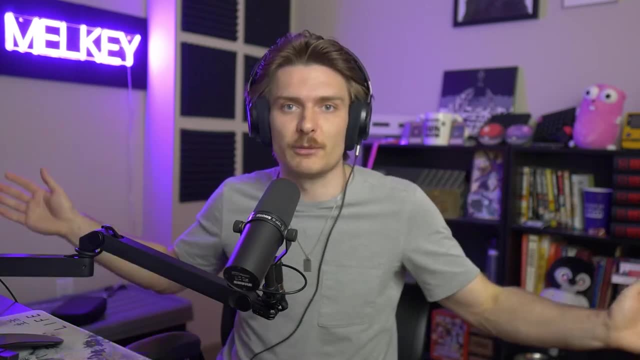 really discover that, huh, this really solved the problem i have. i'm not going to be able to solve it. i'm going to use, and that's perfectly fine, but if you're spending time spinning your wheels on deciding from all the frameworks you see, from a best framework to use in 2023 list, you're wasting. 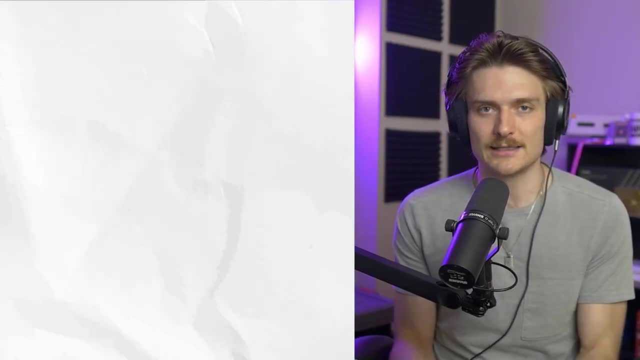 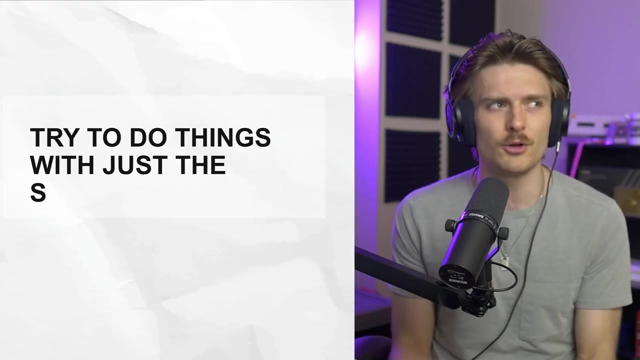 your time. what i recommend to everyone who's starting with go is essentially: try to do things using just the standard library. don't start importing modules or frameworks if you don't need them. they're all the same. but why am i recommending http router, milky? didn't you just 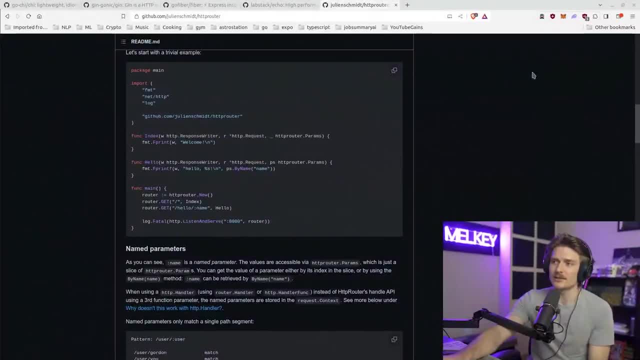 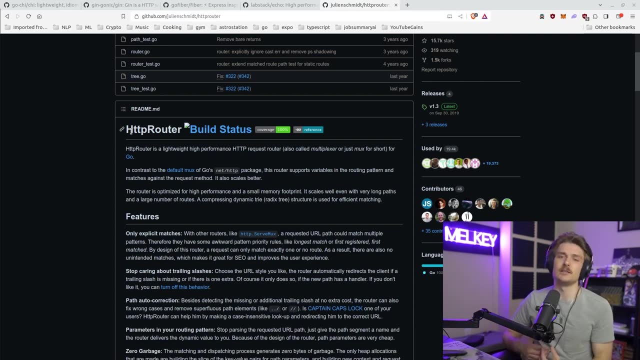 say, try to make it yourself, and that's a valid point. but, like i said earlier, http router is the closest one to the standard library and that is why i personally like it. you don't need to bring anything new. it's simply just a router that gives you everything you need to.